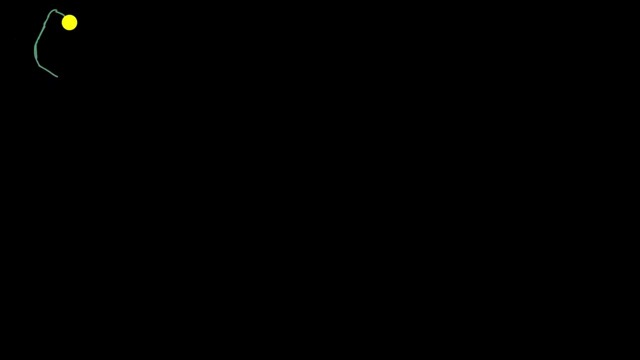 So, as some of you already know, I really enjoy eating a good avocado which, despite its appearance- that it looks like a vegetable but it's actually a fruit. And let's say that I eat two avocados per day, and I eat two avocados per day for six days. 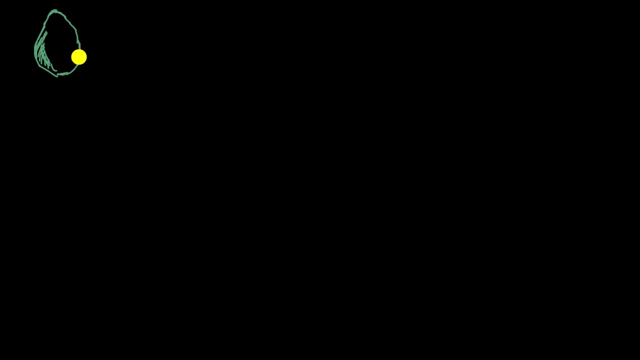 Now there's a couple of ways that I could think about. how many avocados did I eat? I could say, hey, I eat two a day, and I'm gonna do that for six days, So I'm gonna add six twos together. 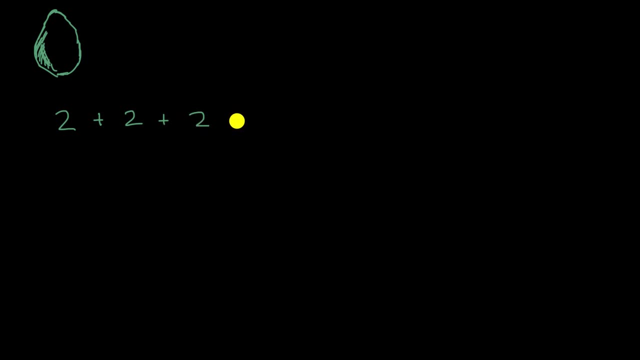 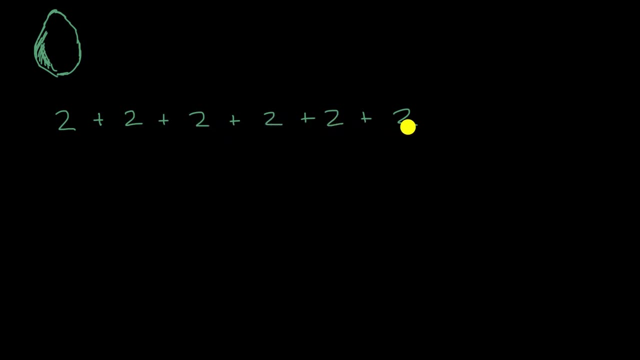 You add another two, you get to eight. You add another two, you get to 10.. You add another two, you get to 12.. And that all is fine. But there's an easier way to express this repeated addition. One way is to view it as multiplication. 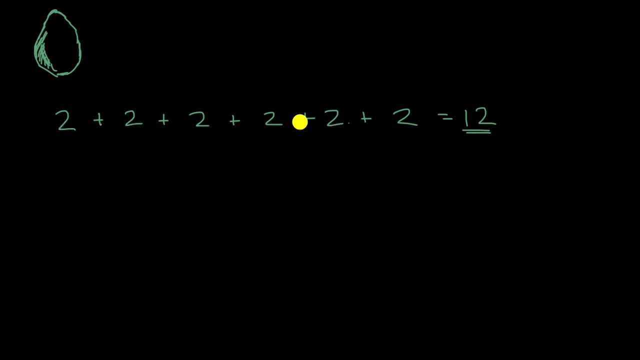 Instead of just writing out six twos and adding them together, mathematicians have come up with a neater way of writing that They'll say: okay, we're going to add up a bunch of twos. How many twos are we going to add up? 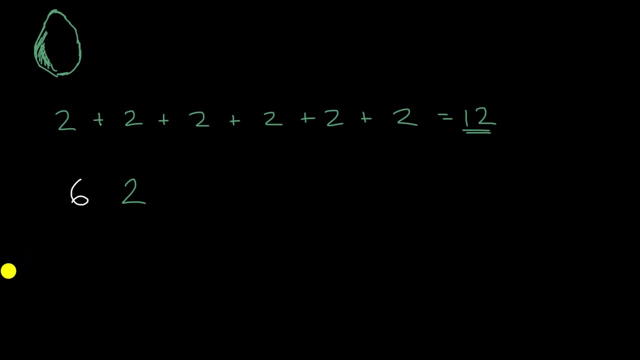 We're going to have six of those twos and we need to come up with some type of a symbol for it, So we will use this X-looking thing, And so six times two can be viewed as repeated addition in exactly this same way. 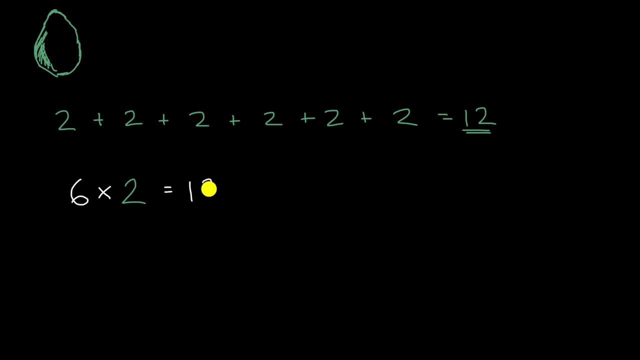 So six times two would be equal to 12. And we could go the other way around. If someone were to ask you: what is four times three? Pause this video and see if you can write it out as repeated addition, like we saw up here. 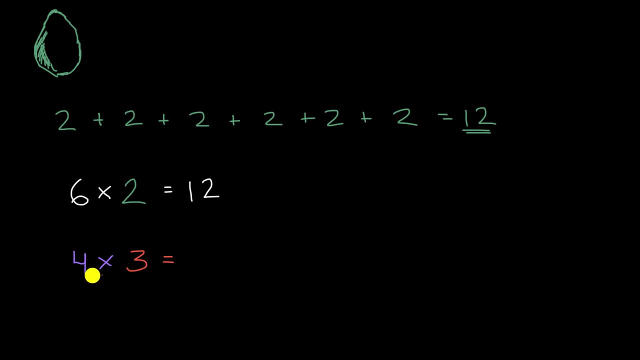 Well, one way to interpret this is to say: this is four: threes. So we could say: this is equal to three plus three plus three plus three, And three plus three is six. Six plus three is nine. Nine plus three is equal to 12..